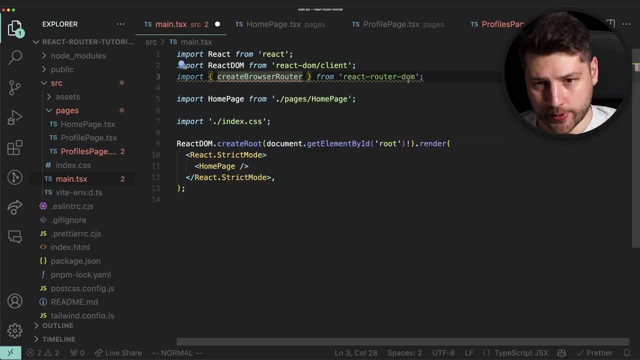 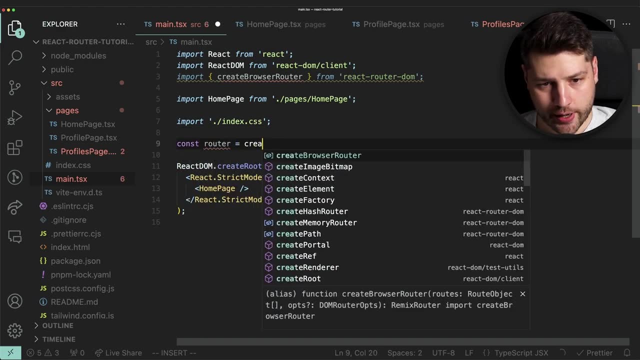 create browser router from React Router DOM, And then we're going to come here and we're going to create our actual router. So we're going to do const router equals, create browser router, And for now we're just going to give this an empty array And later on, 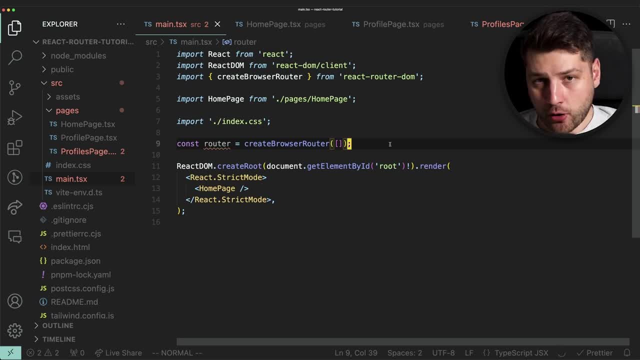 we're actually going to implement our specific routes Now. there are multiple ways that you can create a router with React Router, And this is only one of them. However, this is the recommended way And this is the way that React Router will recommend, if you actually go and look at their 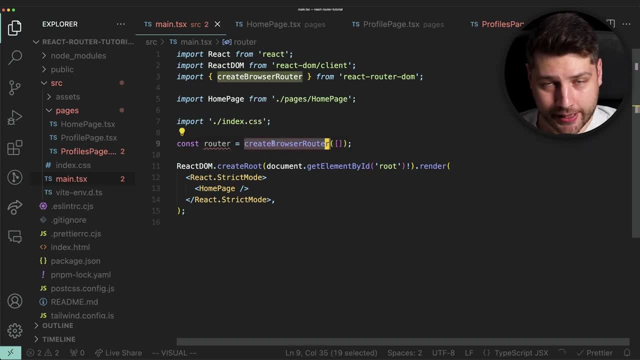 docs. This specific router, the browser router, in 99% of cases is the one that you're going to want to use. This is the one that is exactly like your typical browser navigation. you can go back, you can go forwards between different routes, and your URL is always going to change and is going to. 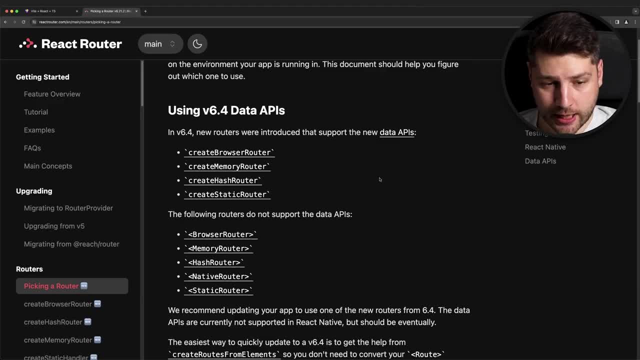 map whatever route you're currently on. But in some cases that behavior is not what the application needs, And in that case you have more options of different routers. you have create memory router, you have create hash router, create static router. all of these serve different purposes. 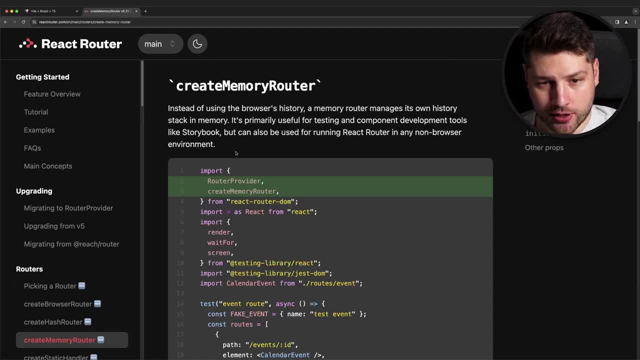 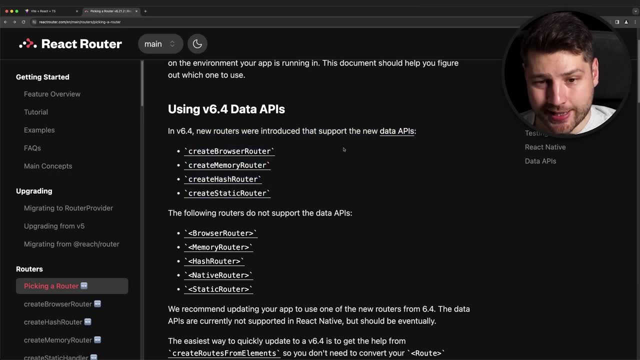 And if you want to use any of them, click here, go at the documentation and see what use cases they are made for. Also, it's important to keep in mind that these routers here are the only ones that let you access the new data API's. stuff like loaders, actions and stuff like that are only 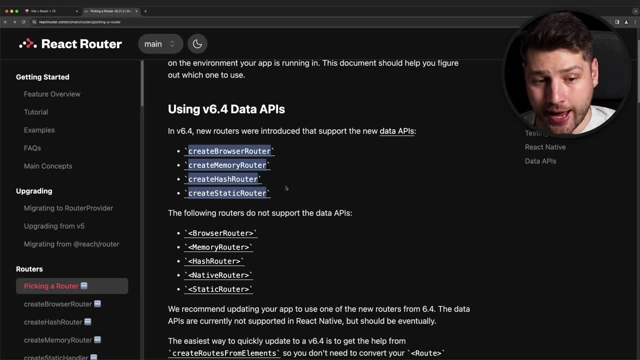 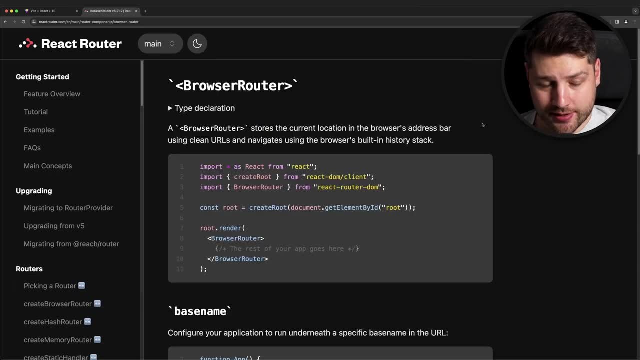 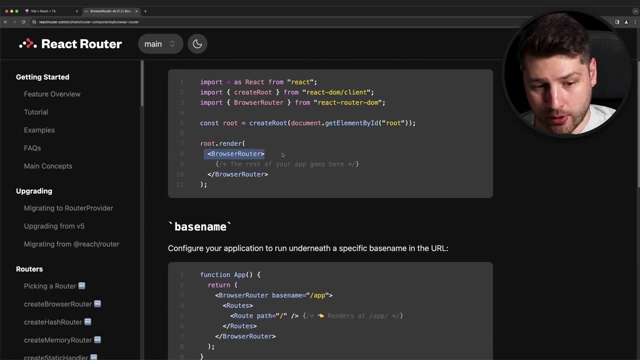 accessible using this API right here. However, you can also create routers using the old way, using these router components right here and declaring your routes in JSX. This is actually the old way of doing things And if you've ever seen react router previously, probably you've seen it like this: you create a browser router and then you declare. 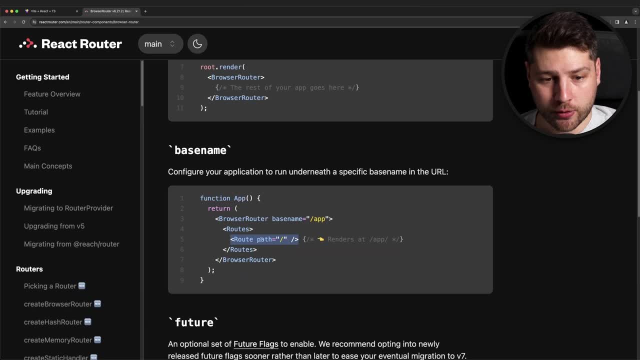 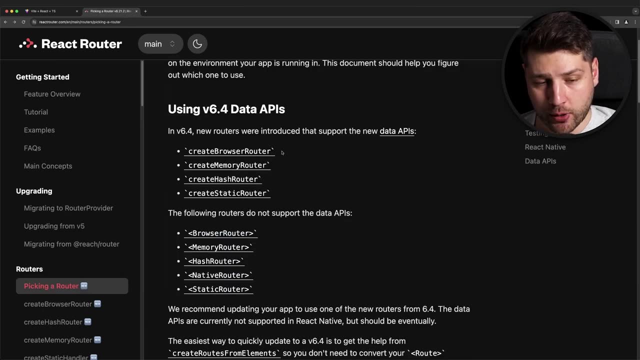 your routes inside of this routes component And for each route, you render a route component with the path, and so on. In this video, however, we're not going to be doing it this way And we're instead going to use the create browser router, As I've just showed. this is the recommended way. 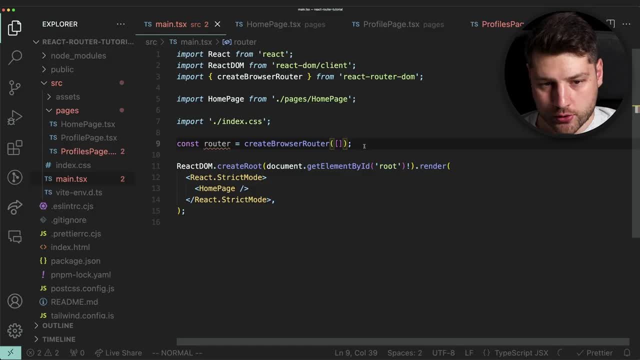 And then we also get access to the new data API's. Cool, So, with that being said, we can now back to our code and continue our implementation of react router. The next step for us to do is to replace this homepage component here that is currently hard coded to render that component. 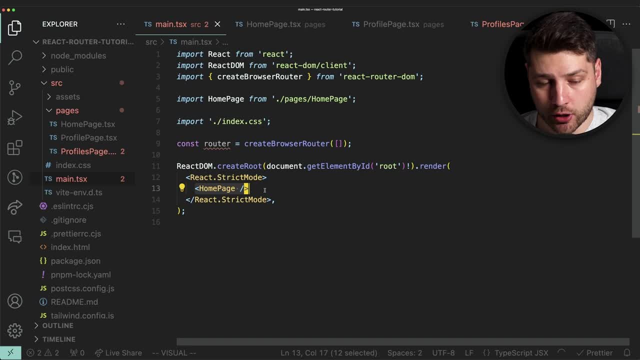 with a router so that we can defer the actual rendering of our components to react router. And for that we're going to need to import the router provider, a component from react router DOM, and plug it into our app. So we're going to come here and do. 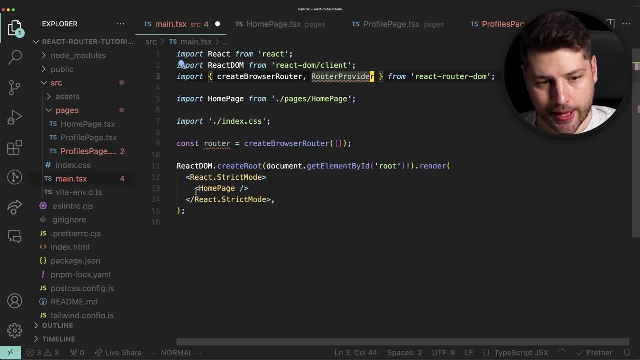 router provider and import this directly, And then we are going to replace this homepage with router provider And we're going to pass it or router like. so What this is going to do is that now we've deferred the entry point to our application to react router and using this router. 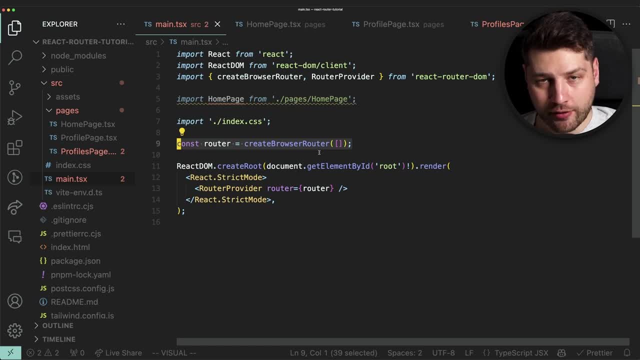 here, which we're going to configure in just a moment, we can actually define what components get rendered at each specific path. And also, by the way, this router provider component is built using the context API from react, which, if you're not familiar with context and how it works in. 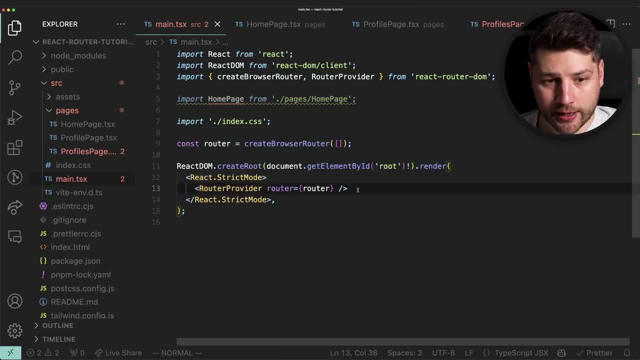 react. I do have a whole tutorial video on react, And if you're not familiar with context and how it works in react, I do have a whole tutorial video on react And, if you're not familiar with context and react context that you can watch to get yourself up to speed. So then the next step for us to do. 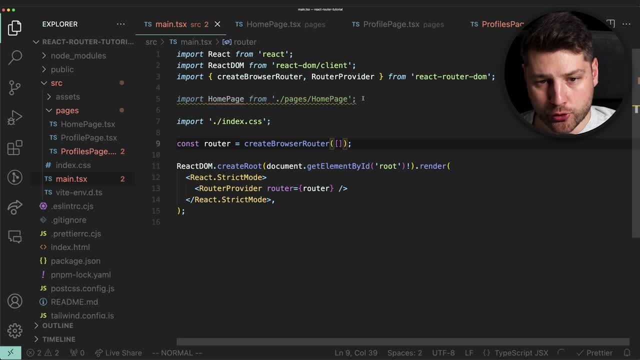 is to actually create a route in a router, And we're first going to start with the homepage. So I'm going to come here, I'm going to create an object for a route And I'm going to give it two properties. The first one is going to be path, And that one is going to be like this: 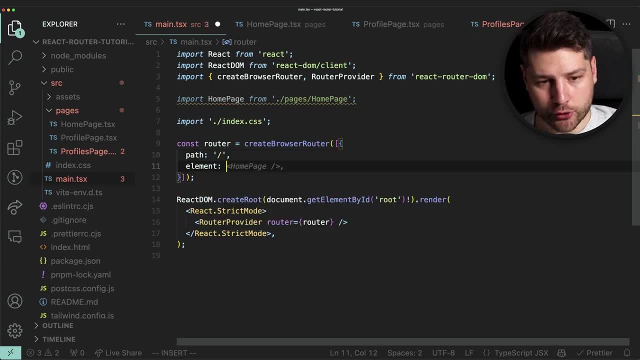 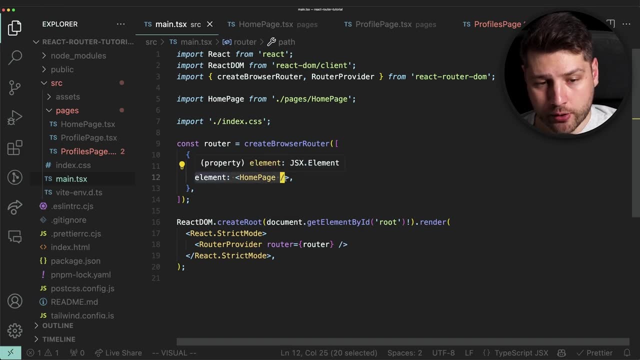 the index and then we're going to give it element And we're going to do homepage like this With this. Now, whenever we are on the index path of our application, react router is going to render the homepage component And I can actually check to make sure that this. 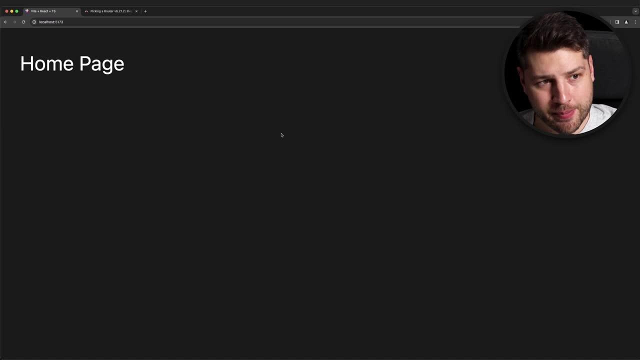 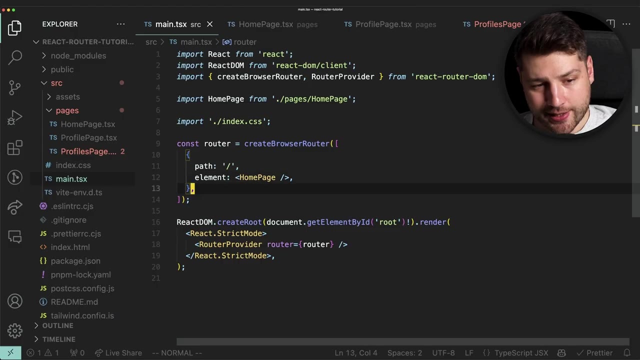 is the case, I can go back to my application, we can go here to our app And then we can reload And, as you can see in the URL, we are on the index page And we're rendering the homepage component. Let's now do the same thing for the profiles page component, the page that is going. 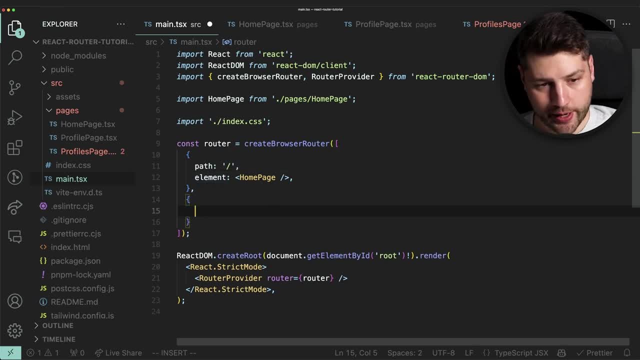 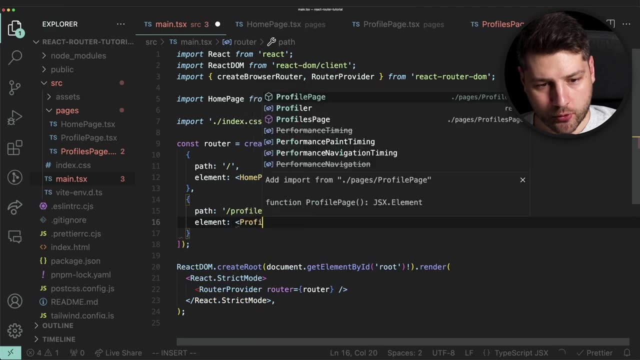 to render all of the user profiles. So I'm going to come here, create a new object, give it a path that is going to be slash profiles, And then the element is going to be profiles page and we're going to import this like this. Now, if I go back to our application, I can go to my URL. 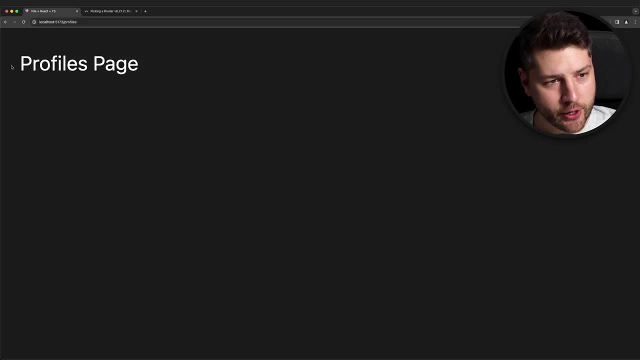 and I can manually change this to profiles, And with this we are now on the profiles page. we validated that our router works as expected. Now here's something important that you have to keep in mind when working with react router, Because this is a URL I can actually change. 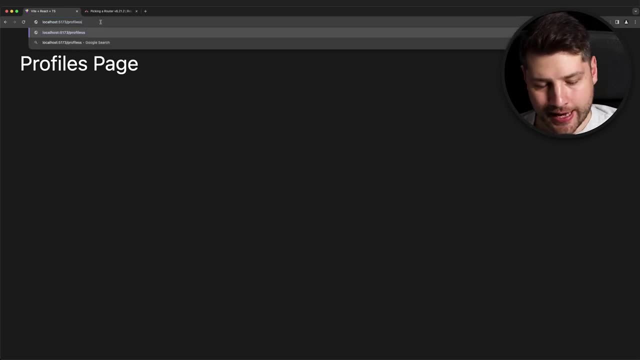 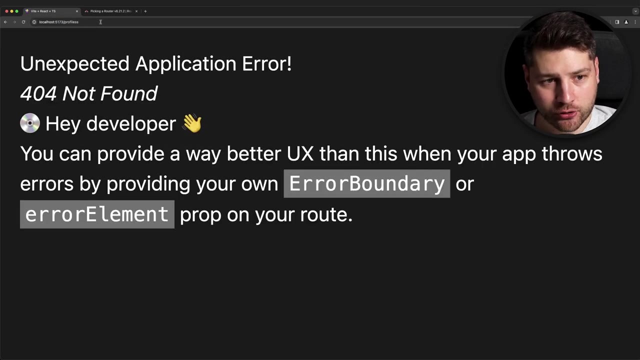 and put anything I want in here. I can add an extra s, And if I add an extra s now, we're going to go to a route to a URL that does not map to any component. If I press Enter, we get here an error message, And ideally. 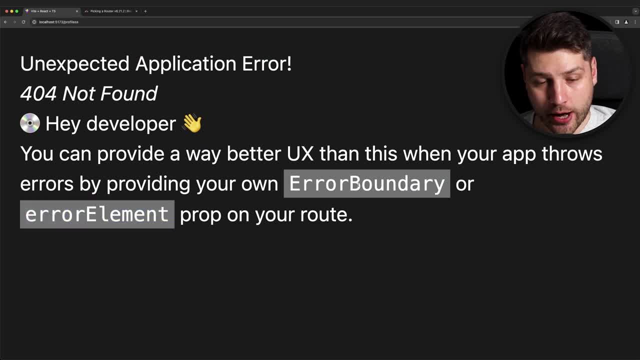 you actually want to implement your own error element or your error boundary to show something different, in case you have a 404 page, just to make it a better user experience for users, And the way that you do that is you come back here, to where you have your router. 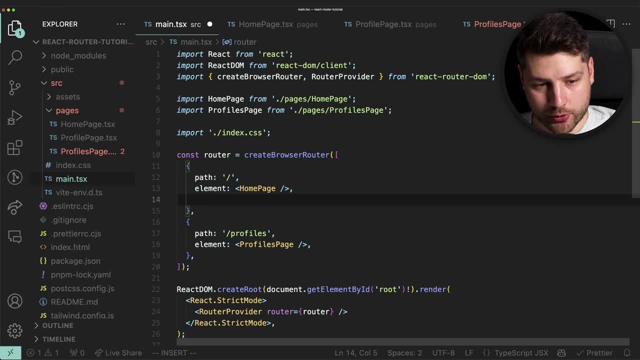 defined And below element you can add an error element. So we're going to do error element And for now we're going to do 404 not found in a simple div. Now if I go back to the application, we're going to see that we have 404 not found. this is our own custom component. I can put any. 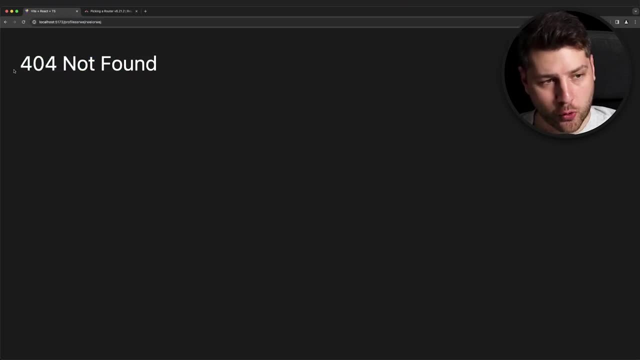 path in here that I want- And it's always going to render this 404 not found- which is a better user experience. Now, this is great, But we can actually take this one step further. we can further improve the user experience by adding a button here that can send the user back to home. 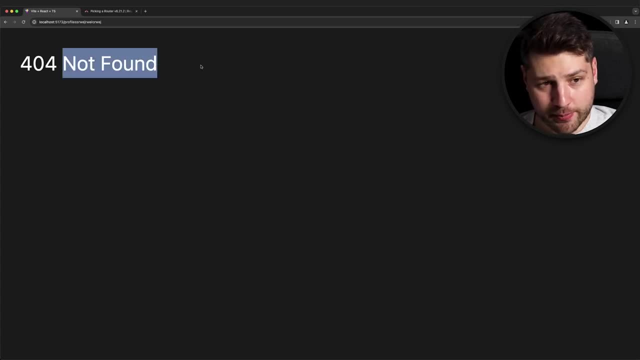 back to a page that is found, Because if a user gets to this page, we can actually consider them as lost, right, they're not supposed to be here, But currently not offering any way for them to find their way back. So having a button here that takes you back. 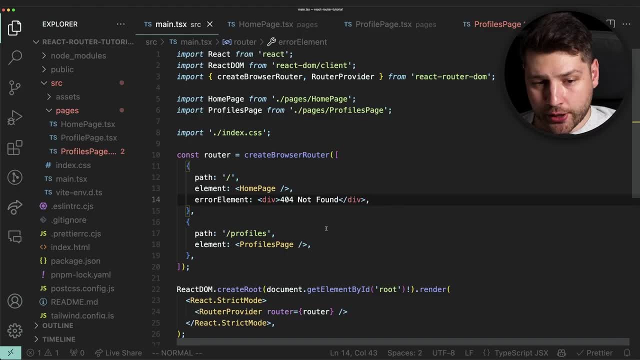 to the index page is a great way to solve that. So the way that we're going to do that is we're going to come here and take all of this code that renders the not found page and we're going to turn it into another page component. So we're going to come here to our pages folder. we're 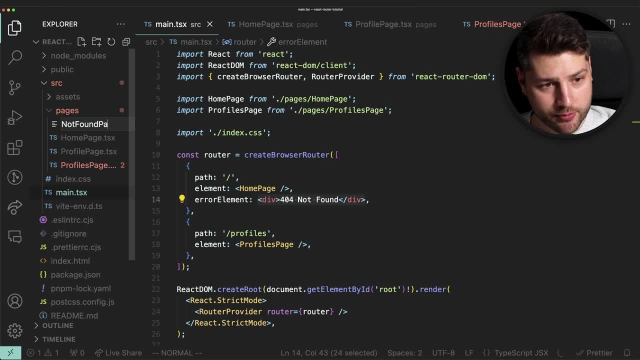 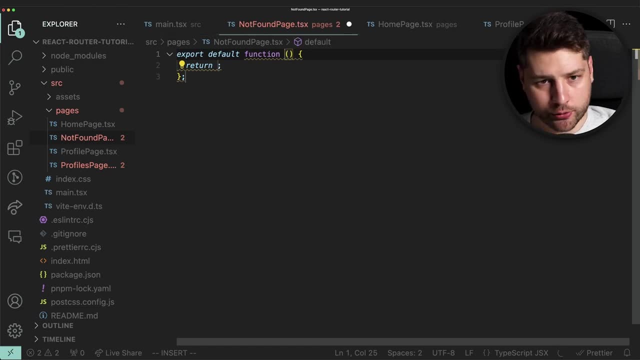 going to create a new page. we're going to call this one not found page. that is x. then I'm going to do here RJS FC and it's going to create for me a component. we're going to do not found page. And then for the actual thing that we're rendering, well, it's going to be the same thing. 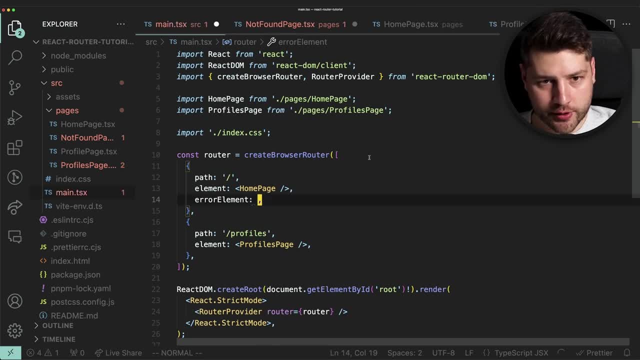 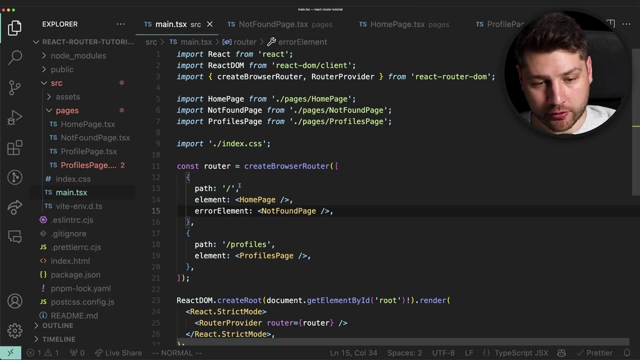 here. I'm just going to take this whole thing like this: remove it, come here to not found page and paste it like so And safe. then we can go back to main and actually put the not found page here. So we're going to do not found page and then render it like so And now we've converted. 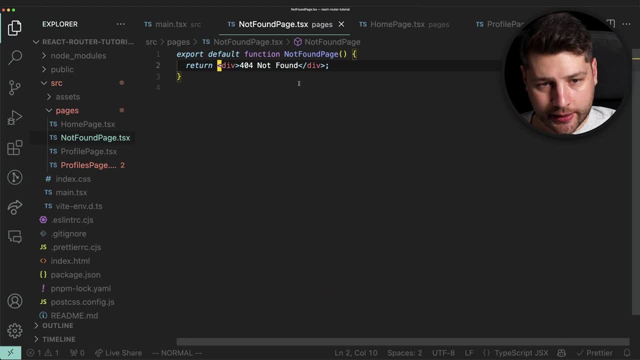 our custom code into a custom page component, And here in this component is where we're going to implement our link back to home. So we're going to go back to our page and we're going to go back to the homepage. Now, in React Router there's a specific way to handle links you don't. 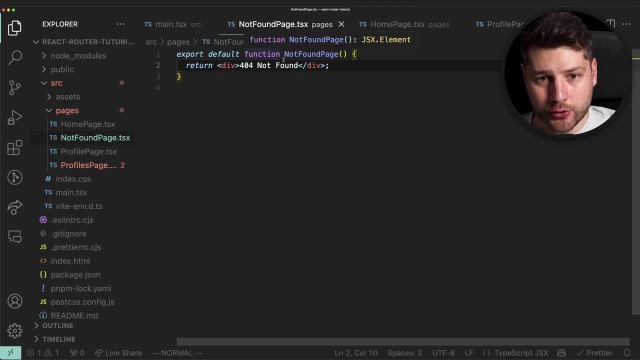 use an a tag and anchor tag directly, you actually use the link component. So let's come here at the top And let's import link from React Router DOM And actually I'm going to show you the differences between link and a normal anchor tag. So we're going to come here and we're going to do two. 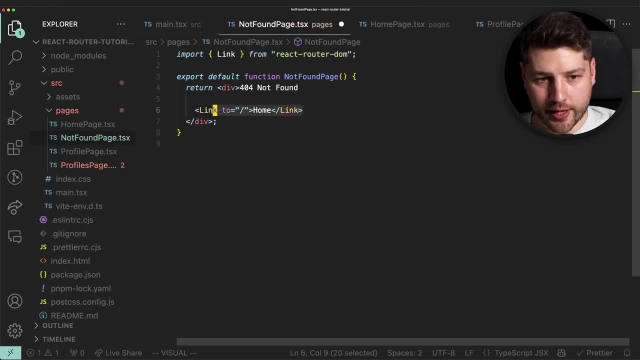 things First, I'll let copilot be very helpful. Yes, this is the way that you create a link using React Router. you create the link component. I mean you use the link component and then you give it a to property, And this is going to be the path that you want to actually redirect to. 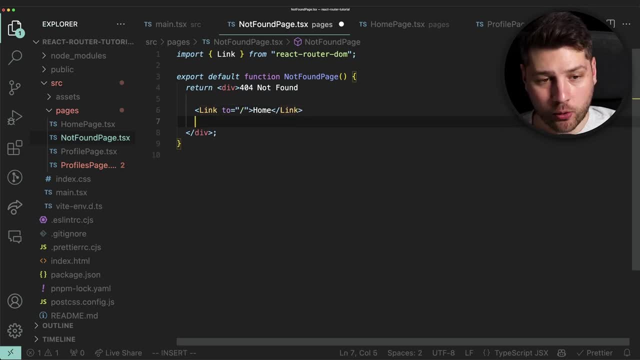 And then right below I'm going to do the same thing, but now with a normal a tag. So I'll come here, I'll do a and then h ref home, And then we're going to put home as well here And actually 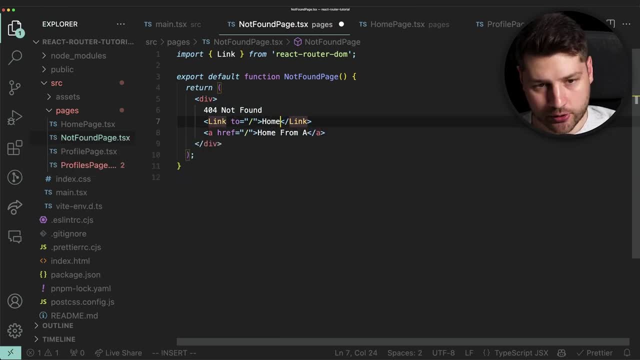 let's put from a and then here we're going to put from link, And actually let's put like this: And also, what we can do is we can add a class name here, we can do flex, flex call and we can do: 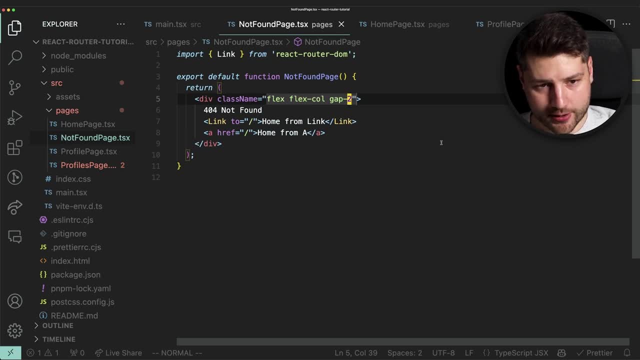 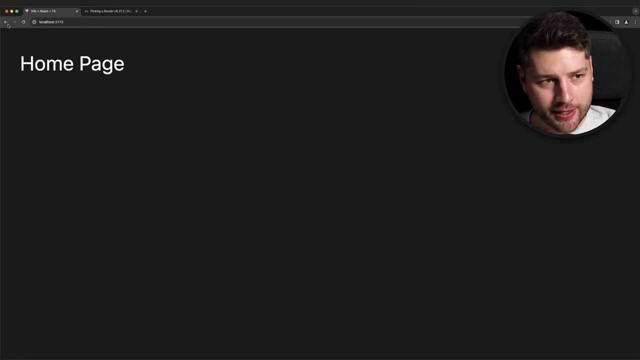 gap To this is going to give us some basic styles. Now, if I go back here, we have our updates, we have four or four not found from our custom component, And then we have a link here, home from link and then home from a. if I open up the console here and I actually inspect both, 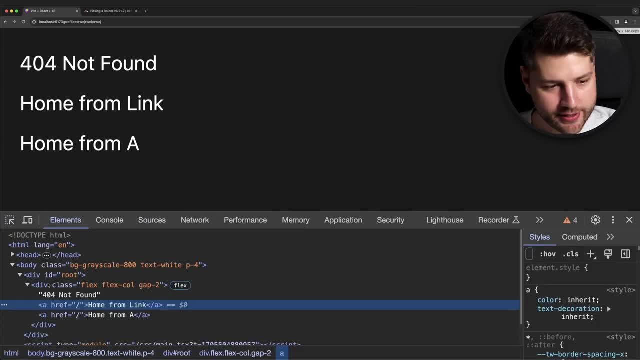 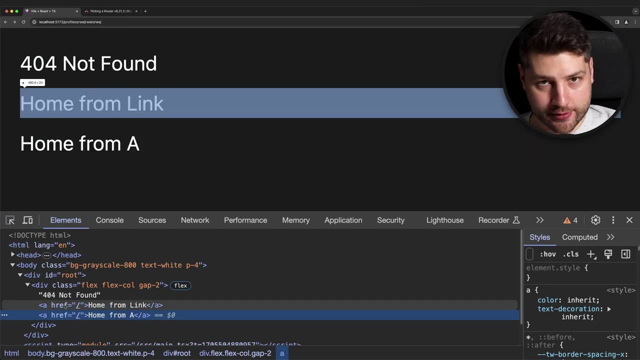 of these. you're going to see that this is an attack right here, if you can see it. this home from link is an attack and anchor tag, But so is this one home from a. they're both anchor tags, So what's the difference? The difference is that this link 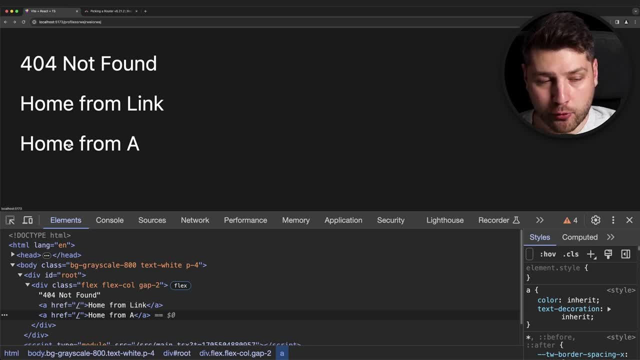 this native anchor tag that we have here is actually going to perform a whole refresh before showing you the new page. This is how links work natively in browsers. you click a link, it opens up a new page, but it does a full page refresh and it requests the whole HTML and. 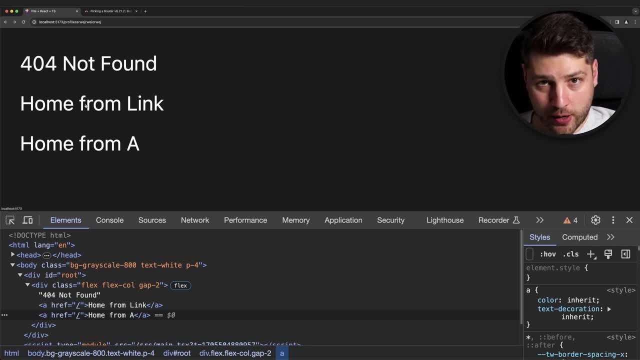 JavaScript all over again, compared to this, a tag which comes from the link component from react router. this is not going to refresh the page at all And this is actually going to perform client side routing. it's going to navigate the page using JavaScript, and JavaScript only. 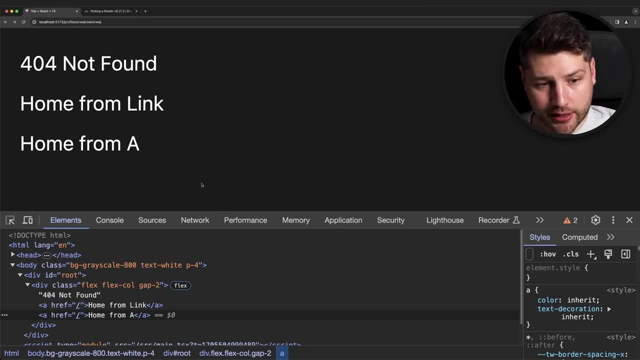 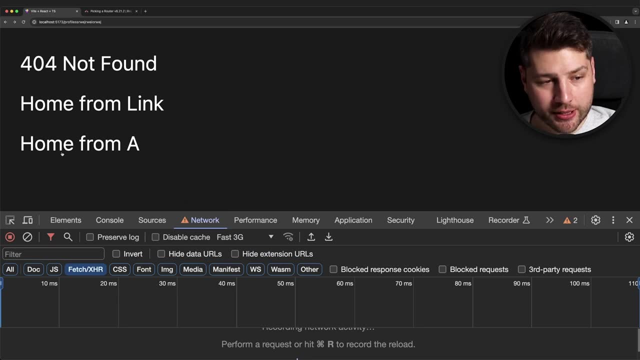 without refreshing the page, And you can actually see this if you click both of these links. So let me first go to my network and actually slow down my network So that you can actually see what's going on. I'm going to click home from a and you're going to see that the browser reloads. 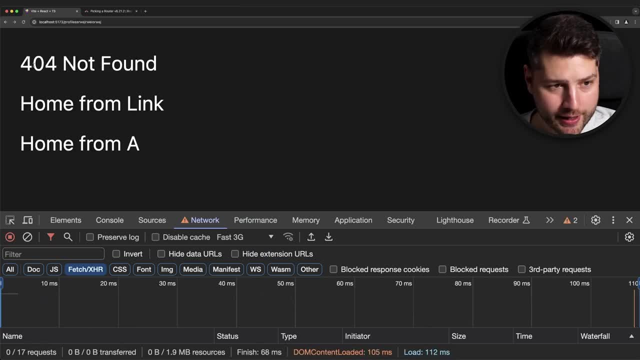 everything is fetched again from scratch. then if I go back and I click home from link, you actually see that the transition was instantaneous and we did not refresh and we didn't load any extra data. This is what react router does. it does client side routing. 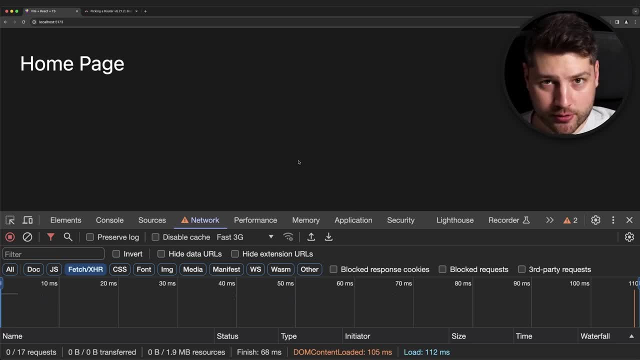 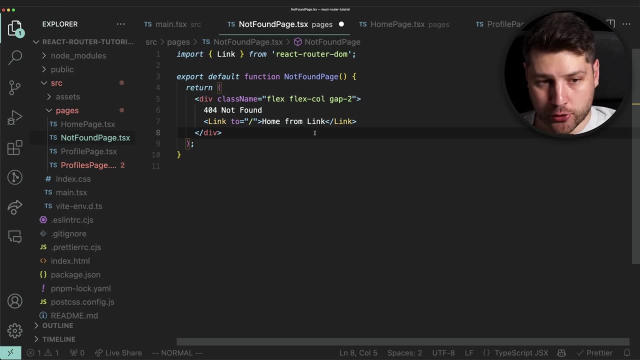 script only, and it provides a much better user experience. So now with this we're actually done with the not found page. we can maybe just remove this a tag here so that we don't allow our users to click it, And we can just leave this link from react router. 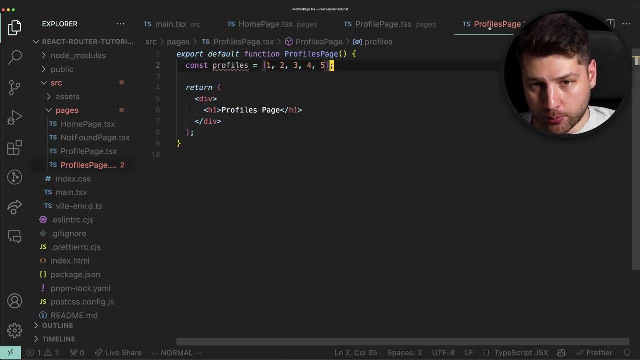 we can close this page And now we can start to deal with the actual profiles page and seeing an individual profile. So the first thing that I want to do is actually want to render out some links for the profiles page, because currently the profiles page only shows this. So I'm going. 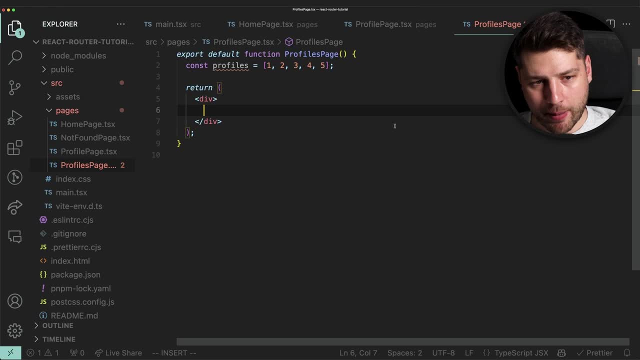 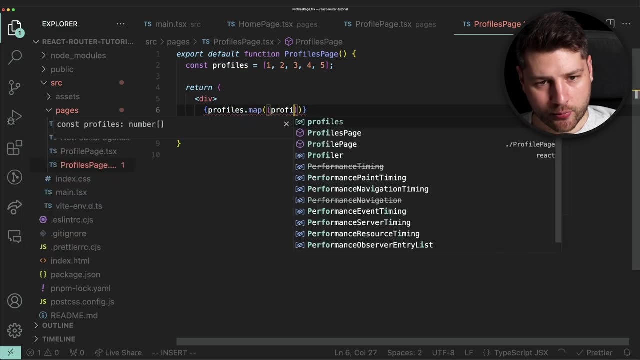 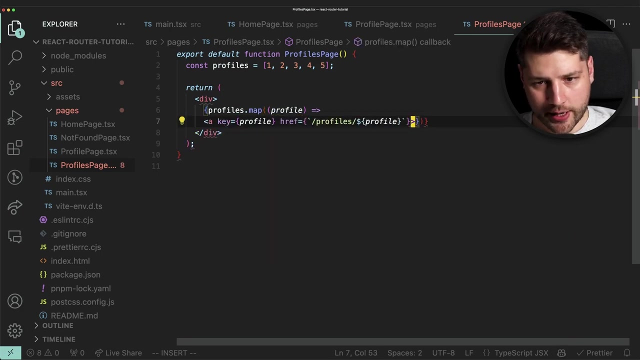 to remove all of this here And instead I'm going to use this profiles and map over them and render a link for each single profile. So we're going to come here and do profiles, dot, map profile and we are going to return a key that's going to be profile and then href profile And 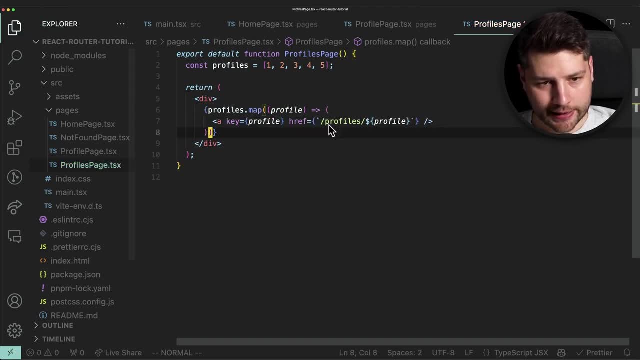 let's see what is wrong here. we don't have this, And there we go. Now, for each profile, we're just rendering an a tag, And actually this should be a link tag, because we want to have client side navigation. 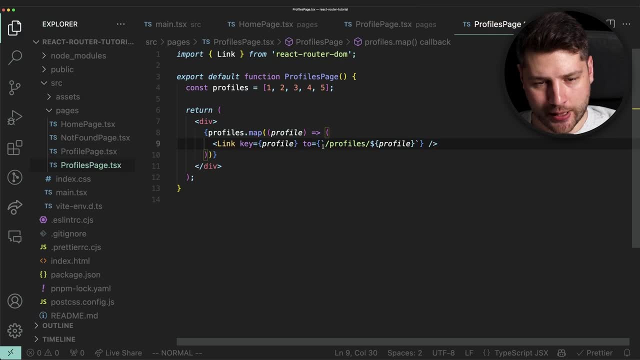 So we're going to render a link And instead of href this is going to be two, And each profile is basically going to link to slash profiles, And then we're going to put the actual ID of the profile in the URL. And actually I just realized that we have to actually put something. 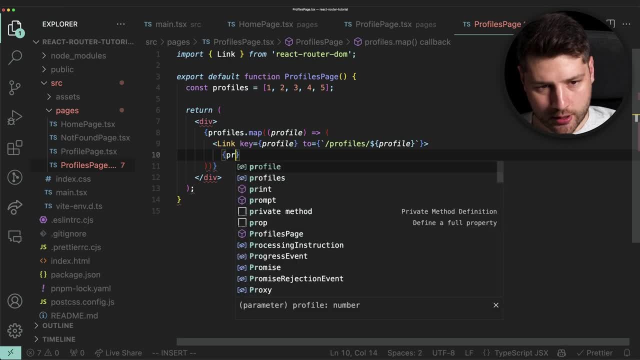 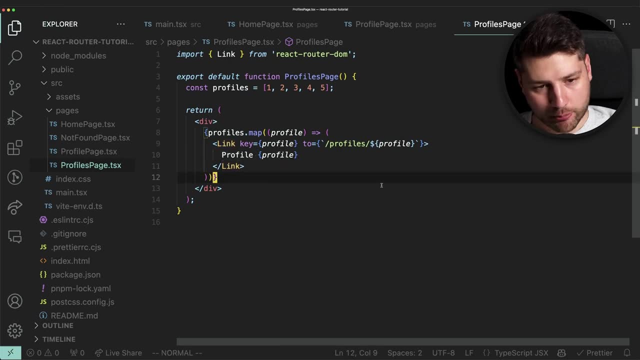 in the link. we have to give it some text. So we're going to do here profile, profile and and we're going to close the link like: so now we would actually be able to see something on that profile. Then if we go back to our application and we now change the URL to: 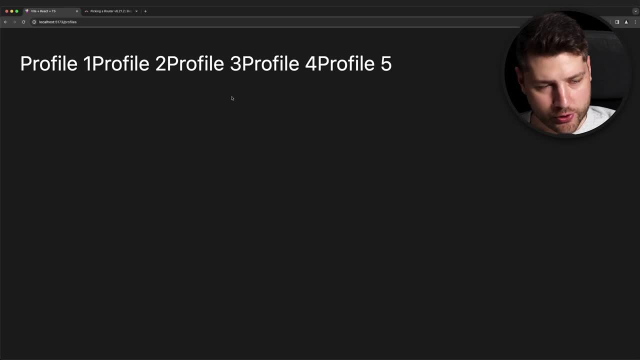 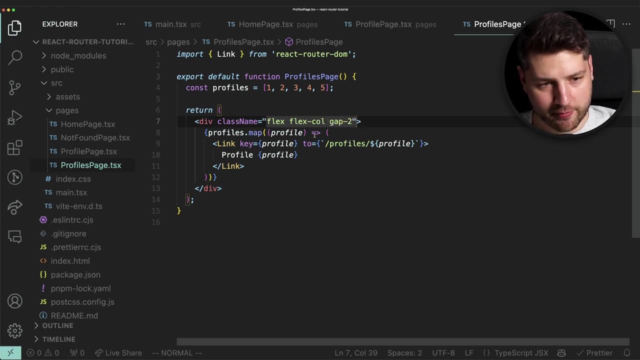 profiles. we now see all of our profiles right here, which is great. Maybe we want to come here and just do something like class name, flex, flex, call and then gap to, just so we have better styles And there we go. This looks a lot better. So now we have five profiles, five different links. 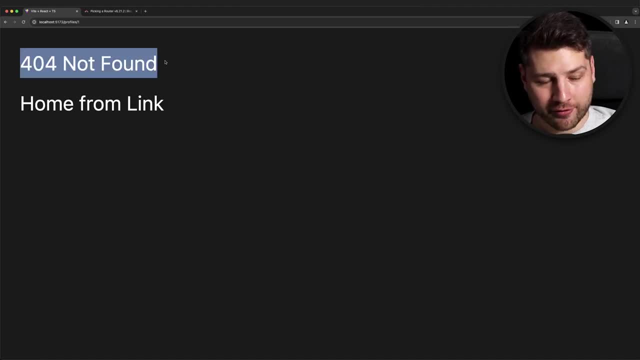 But if I click any link, we're actually sent to the 404, not found page, because we haven't yet implemented the single individual profile route in our app. So let's implement it. Let's come back to our code And let's come here to our profile. And let's go back to our code And let's come here. 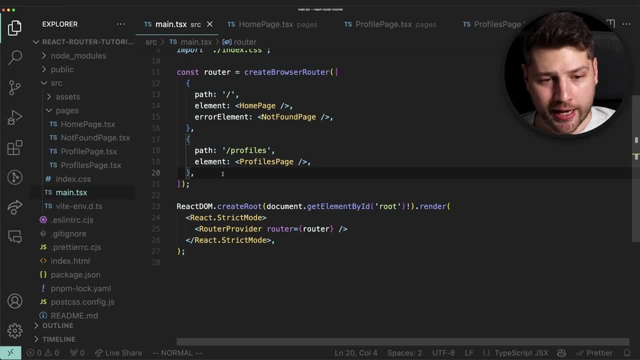 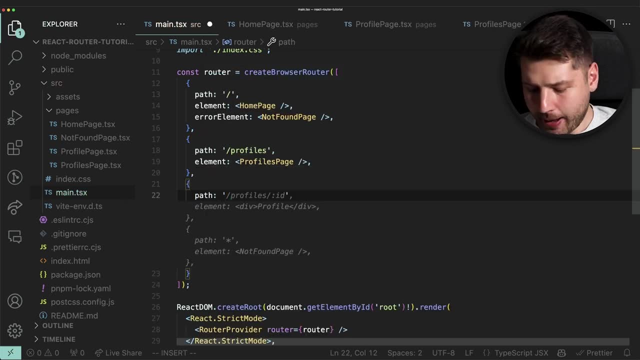 to maintsx. Here we have to create a new route, and this time for the profile page of a specific profile. So I'm going to come here, I'm going to make path. And now for the path, we have to ask. 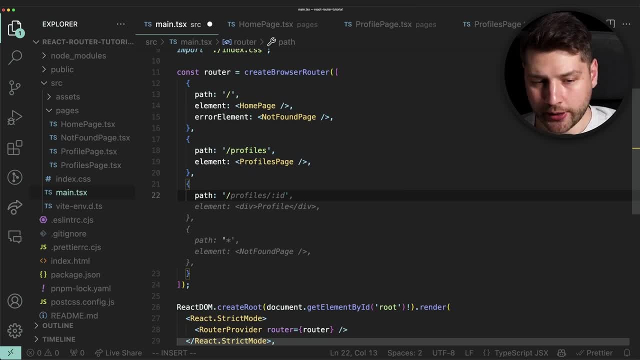 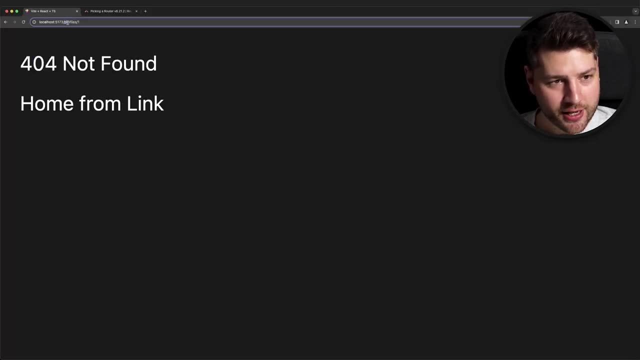 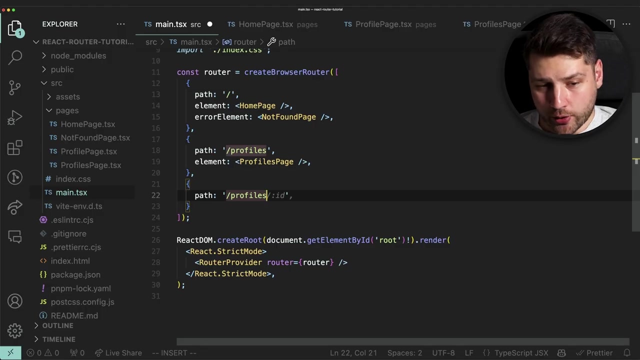 ourselves the question: what path do we actually want to do? we know that it's going to have to be slash profiles, But how do we actually get if you see here in the URL we have slash profiles, slash one- this is a dynamic parameter that can change for a specific profile And in react router. 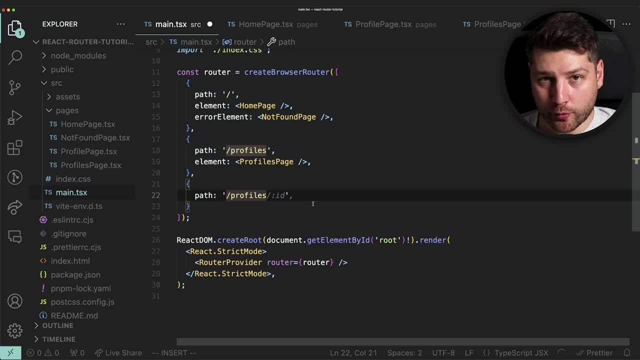 there's actually a way to implement dynamic paths to put some sort of property in a URL that can change based on the specific entity And, as you can see here, copilot already knows exactly what I'm going to do. The way that you do that is: you do this, you do slash for a different part of the. 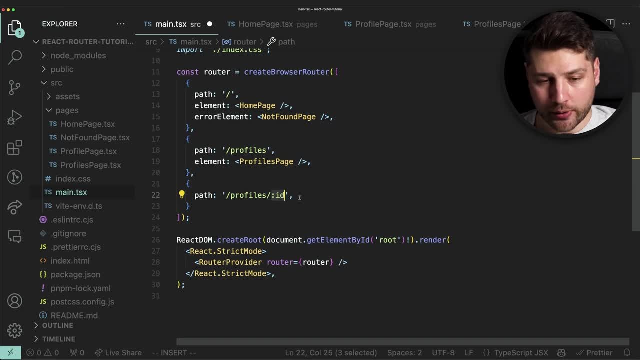 URL And then you put colon and then the actual property here And what we're going to do: instead of ID- because you can name this any word that you want- we're going to do profile ID, because this makes it just a little bit more clear What this is going to do. 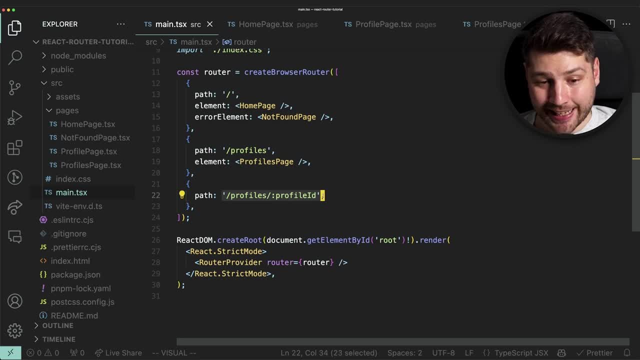 is it's going to tell react router that this URL has a dynamic parameter And this part can be different, it can change, it can be one, it can be two, it can be three, it can be a, B and C or it can be anything. this is dynamic And anything that matches this pattern here. 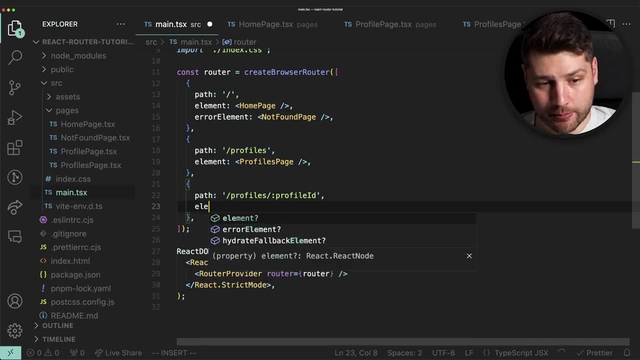 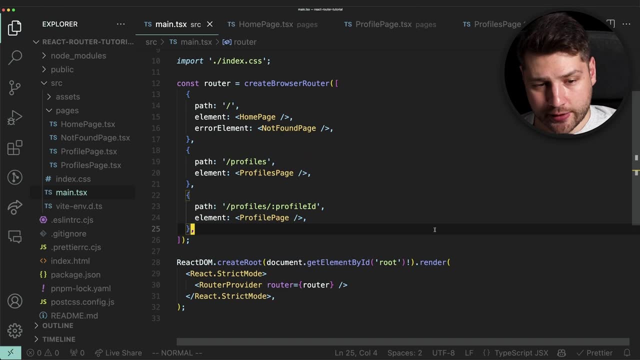 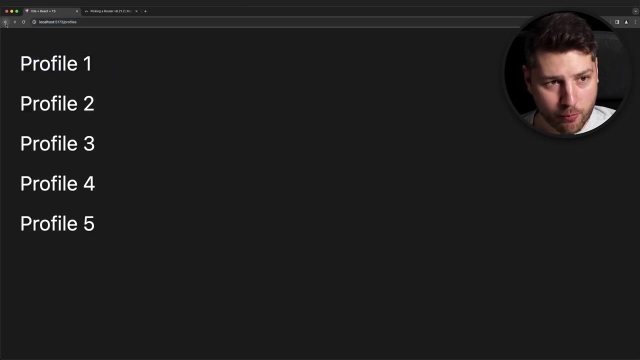 is going to render out the actual element, which, in our case, is going to be the. what is it? the profile page, singular, like so. So now with this, if we go back to our application, we actually see profile page being rendered on slash profiles, slash one. if I go back to where we were before, 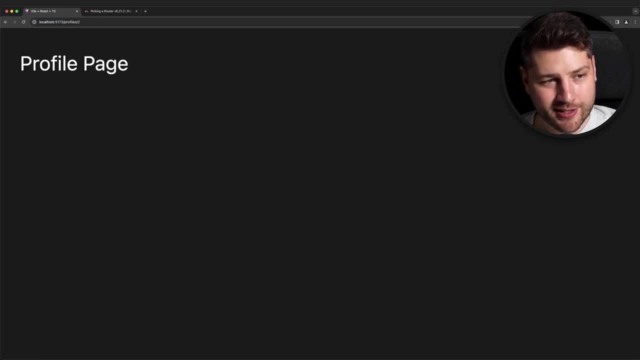 we have profile 2345, I can click any of these profiles And it all puts me to profile page. you can see here it's two. if I go back I click three. in the URL it's three. all of these match. 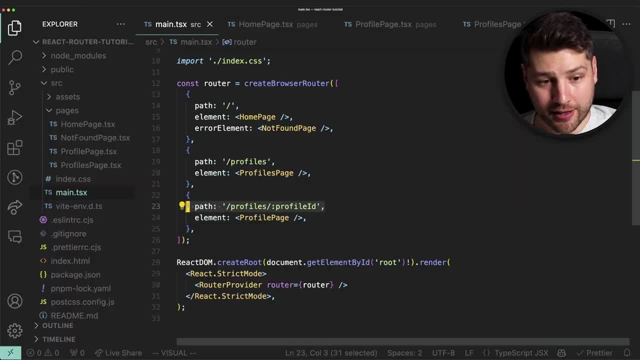 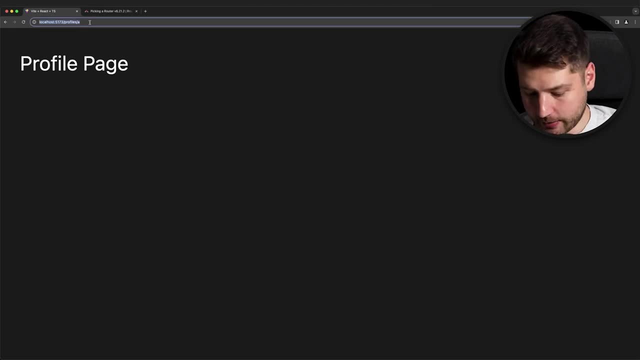 the profile page, because that's what this means, That's what this path here means. it can be anything. I can go back to the application And I can change this to a, for example, and it will still work. I can put here any random. 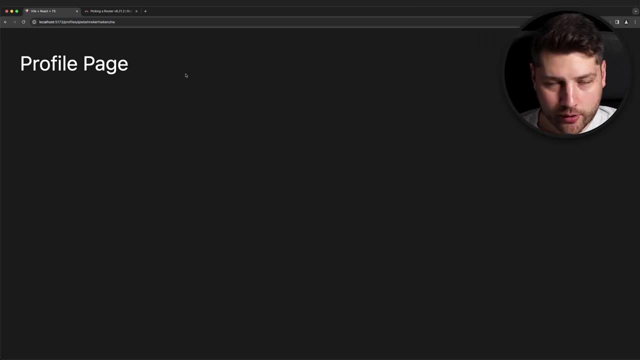 characters and it is still going to render the profiles page. Now, if you're observant, you'll actually notice that there's something missing in this page, this profile page. this component doesn't have context, is not aware of the actual profile ID. that is currently. 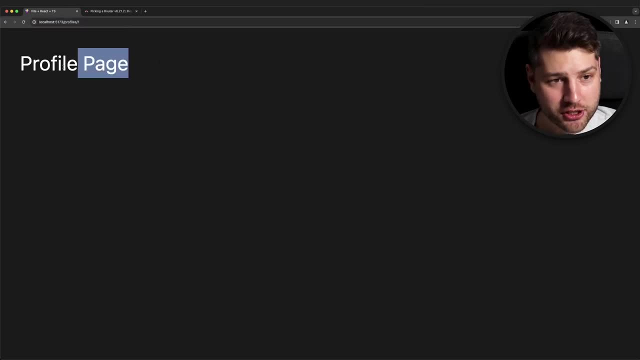 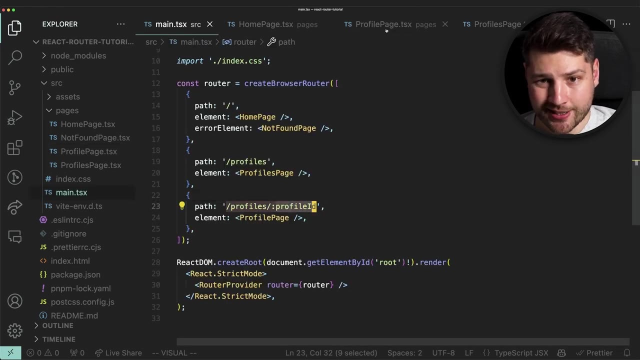 rendering. I can change this to anything and nothing is actually changing on the page. what we need to do is we need to make this component aware of this parameter right here, because in a real world application, if you have a profile page, you want to know the profile ID. 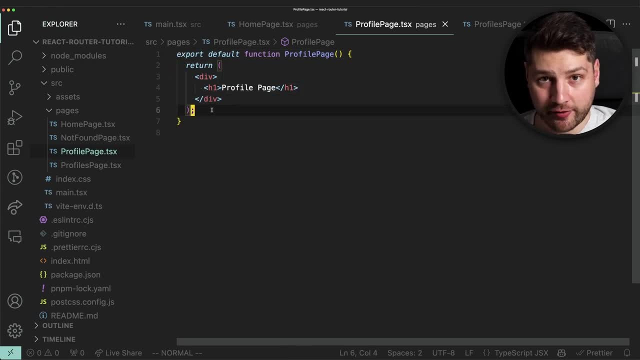 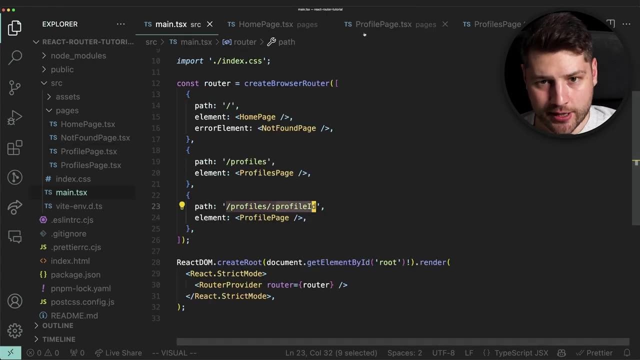 because you're going to want to use it inside of this component, maybe to fetch the actual profile data of that specific user And in react router. the way that you access these parameters right here is actually quite simple. you make use of the use params custom book. So we're going to come. 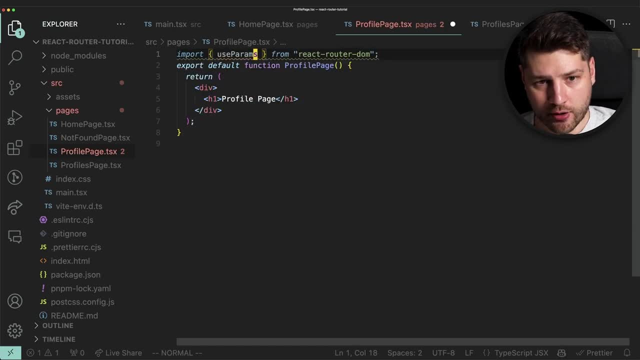 here: import use params from react router, And then we're just going to do use params, call it like so, and this, this use params, is going to return you all of the parameters available of the specific page. So we're going to go ahead and create a new page and we're going to create a new. 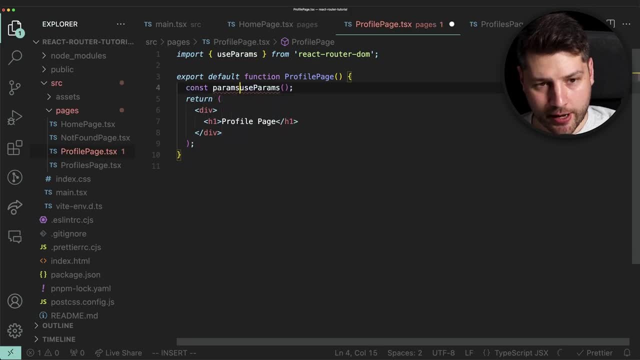 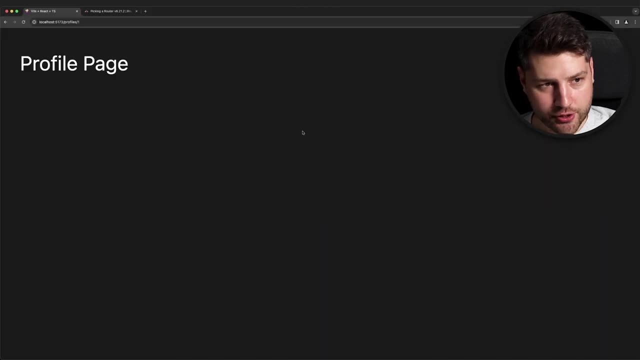 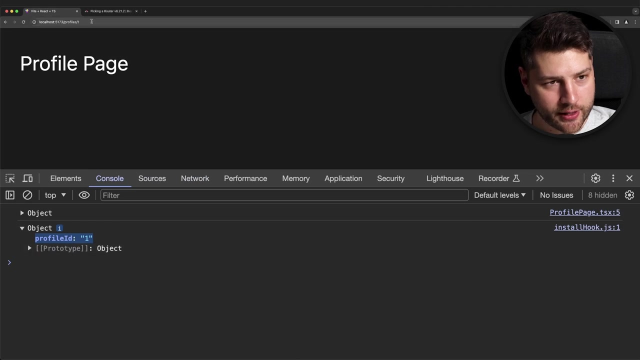 page. So what I can do is I can come here, I can do const params And then I can just console dot log params to see what we actually get If I go back to the application and I open up the console here so that we can see we have an object And here we have profile ID And then one. 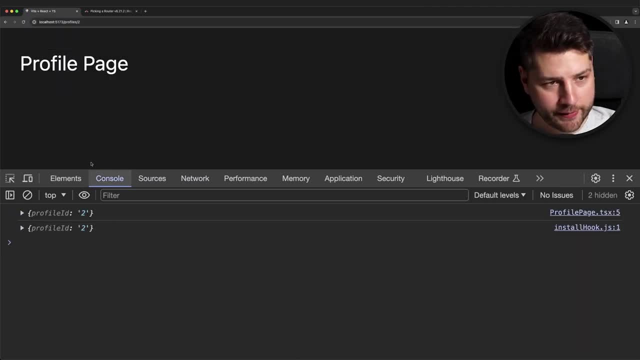 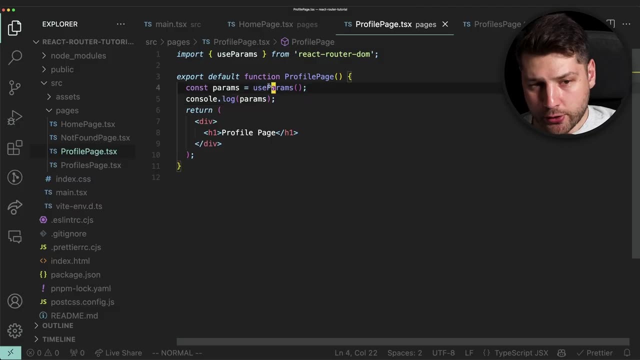 if I change this to two, we get profile ID to. if I change this to any sort of characters, we get profile ID. all of this gibberish- By using use params. we've now given profile page context of the parameters that are available to this route. So now what we can do. 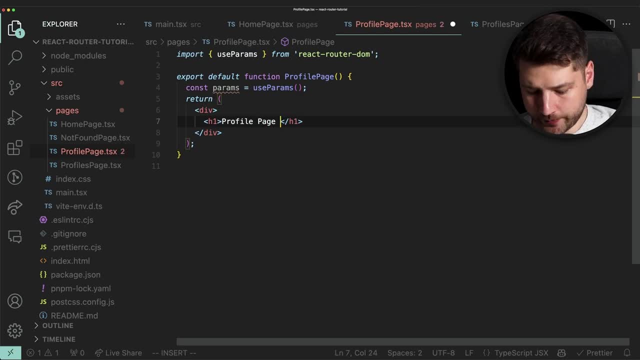 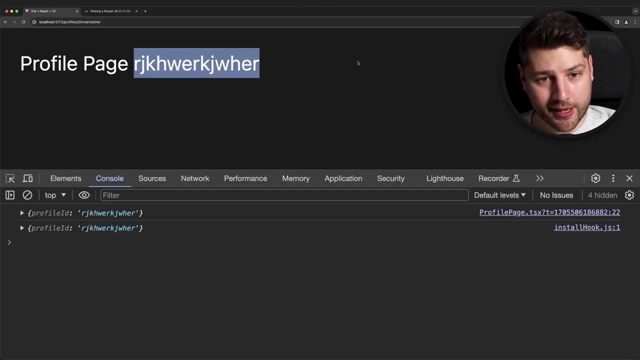 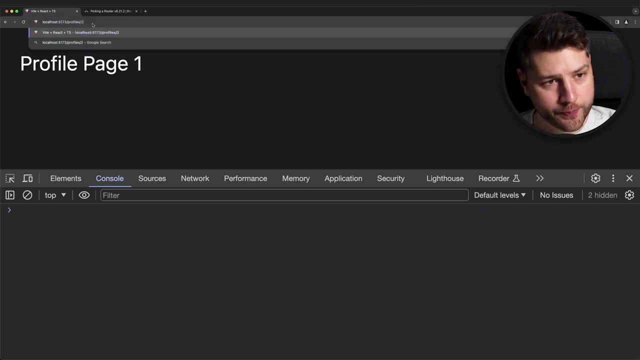 is, we can get rid of this console log And we can just do here: params dot, and this was profile ID. If you close this now, we go back here and the profile ID is actually shown in the UI. I can go back here to one And we're now seeing profile page one. I can go back here to two and we're 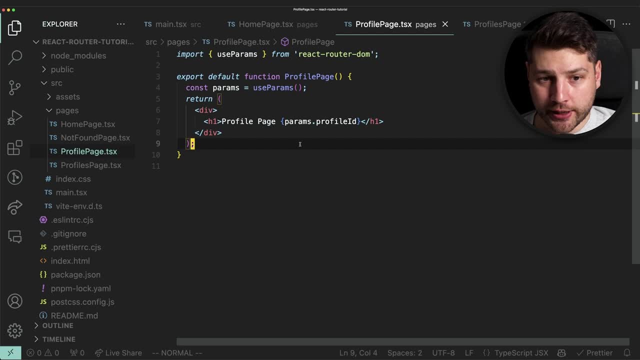 seeing profile page two, you get the idea. Now, if you're working in TypeScript, which we are in this video, I'm going to give you a very simple way to do that. First of all, I'm going to give you a. 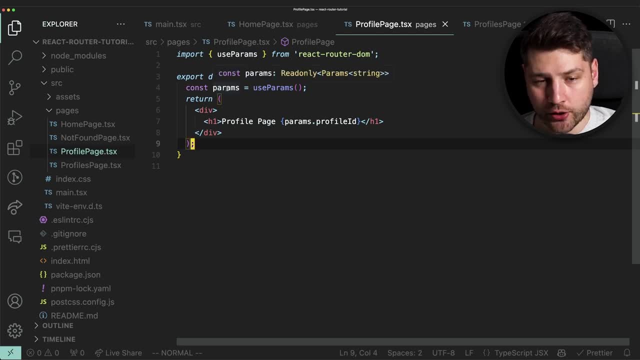 useful tip. As it stands currently, these parameters are not defined. we don't actually know what properties we have in here To fix this. what we can do is we can actually give use params, a type. we can come here and we can put these angle brackets here And we can give. 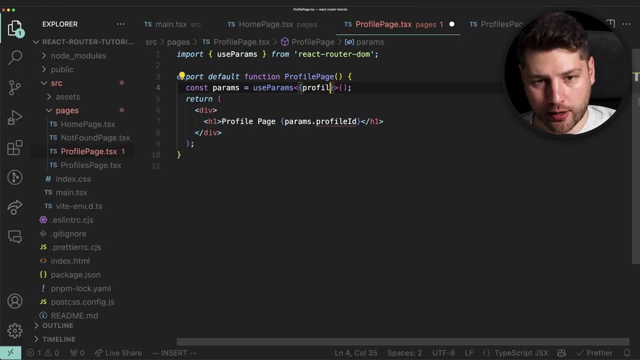 it the type of parameters. For example, we can do profile ID And then we can do this string. Now profile ID is actually going to be typed And if I do here params and then do period, it's going to know that we're expecting a profile ID. 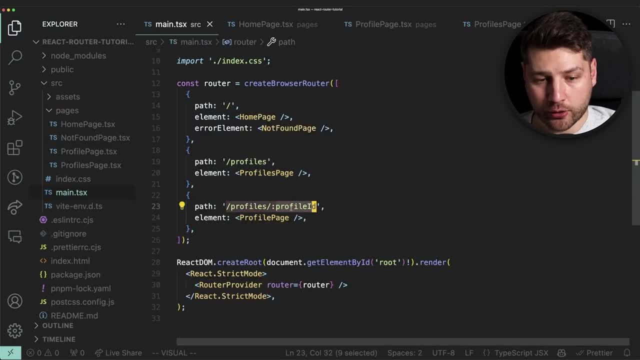 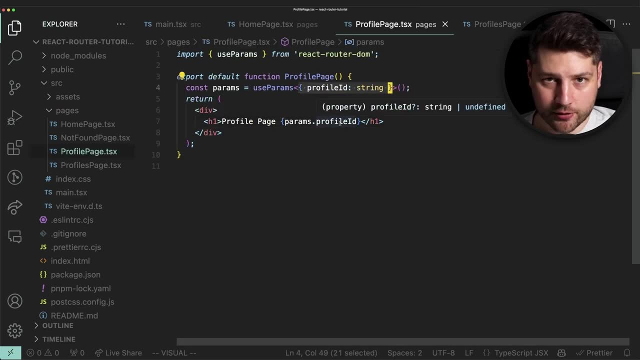 This is very useful in the case where you know what parameters you're actually expecting in this component. you can just give it a type here And then you have automatic type completion in this component. If you're not working in TypeScript, that's totally fine, just skip this. 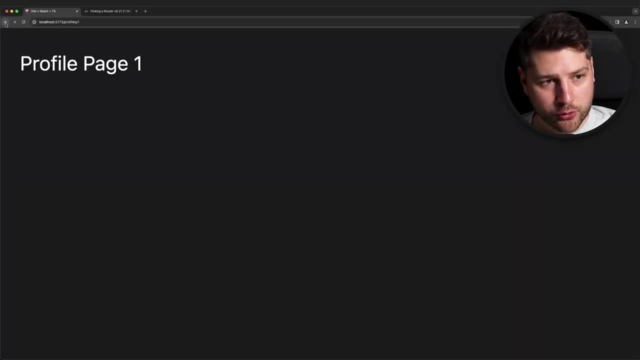 step. It's a small step anyways. So now, if we go back to all of our profiles page- and actually I think it's easier to just go here to slash profiles- I can click profile one. I have here profile page one. I can click profile to profile page two And I can do this for all of our profiles. 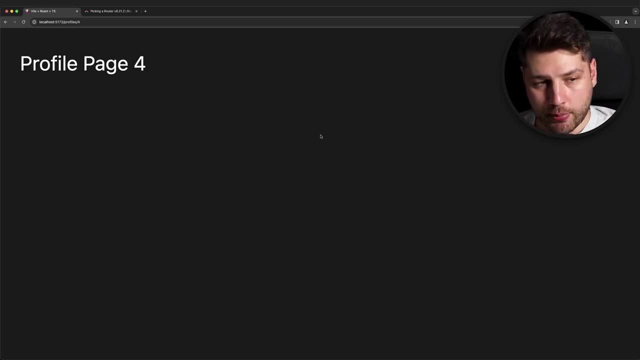 and it works as expected. Now there's one more feature about rec router that I want to show you, that you're probably gonna want to use in your applications The way it stands currently. every time we navigate from this slash profiles page to an individual profile, 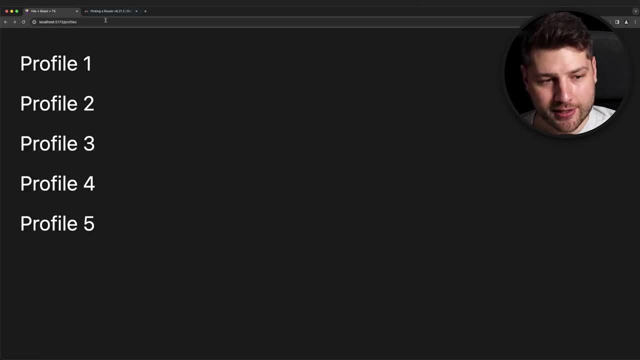 actually rendering all of the profile and we're losing the contents of this page right, Because it is a whole different page. But sometimes in a real world application, you might want to keep all of these profiles here And when you click one of them, you actually only see the profile here and then you can see here, and then you can keep these profiles. I'm just gonna click the refresh animation and then I'm just gonna click the refresh and then you know you're on all these profiles And you can actually see the profiles here, and when I tap this this will show up right here. 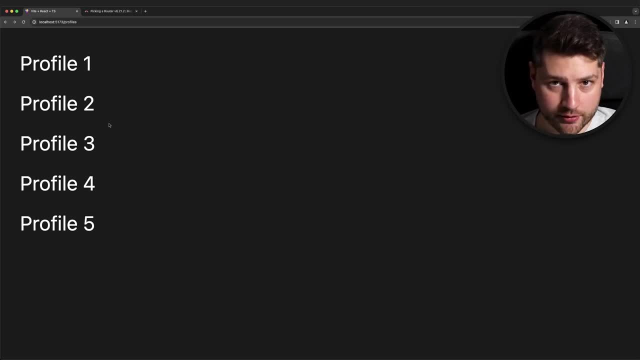 profile on this side of the screen. This remains here on the left And in React Router. the way that we can achieve this is by creating a child root. What we have to do is we have to make this component here, this root, the slash profile, slash profile ID- a child of this root. This way, 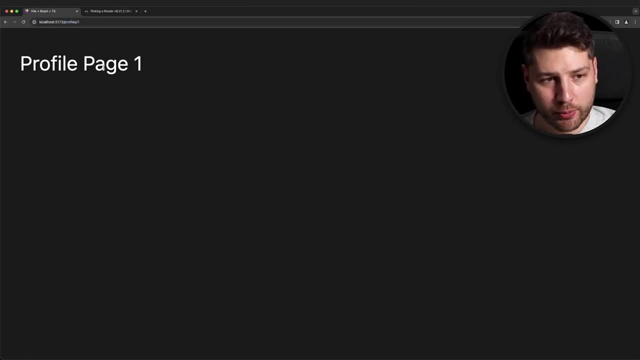 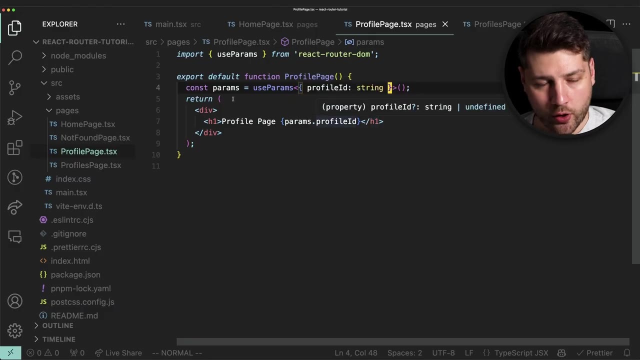 this root is always going to be visible on this path And then, when we navigate to a specific profile, it's still going to be visible here on the left, And we're also going to see this on the right. So, going back to our code, we can come here to maintsx And the only thing that we have to do 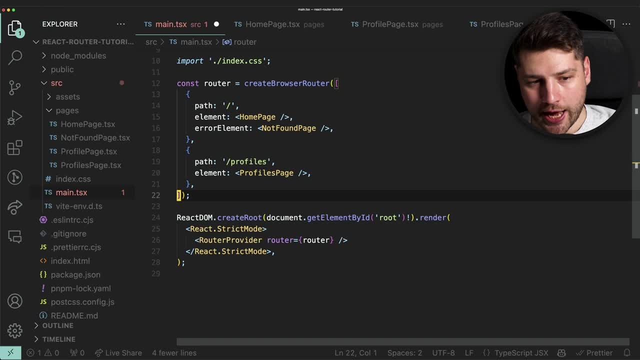 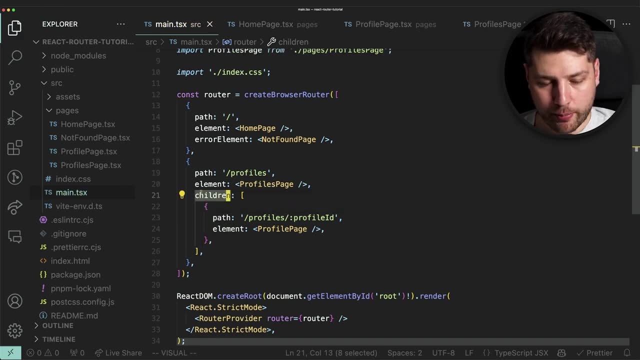 is. just take this path here- the individual profile page- and move it inside of the children property of this root, right here. we can paste it here. This children property allows you to specify some roots that are children of this root, which means that they're going to be rendered. 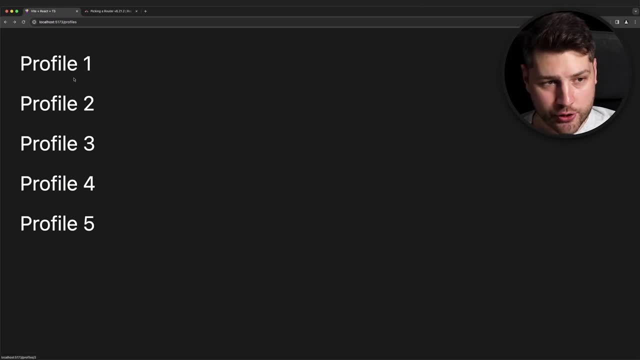 exactly as I've said. Now, if you go to the application, you can click profile one. this root is still visible. The URL here at the top changes. we're on slash profile, slash one, but we're actually not seeing the. 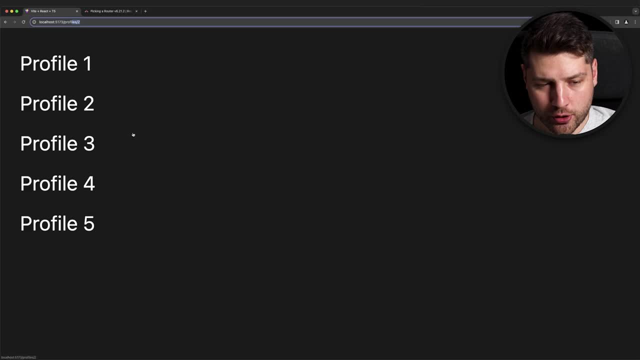 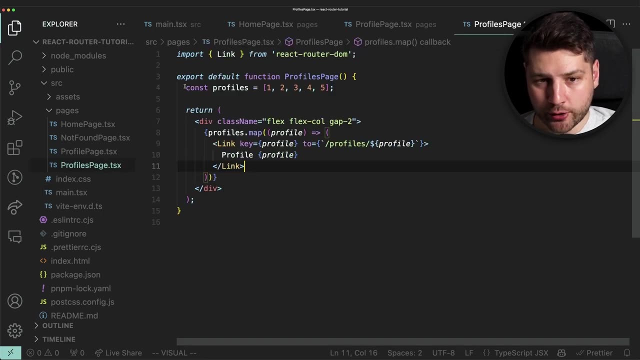 individual profile. I can click to the URL, changes to two, but we're not seeing the actual profile. what's going on? Well, the reason for that is if you actually go to profiles page, that renders all of the different profiles. we haven't told react router where it should render its children roots. 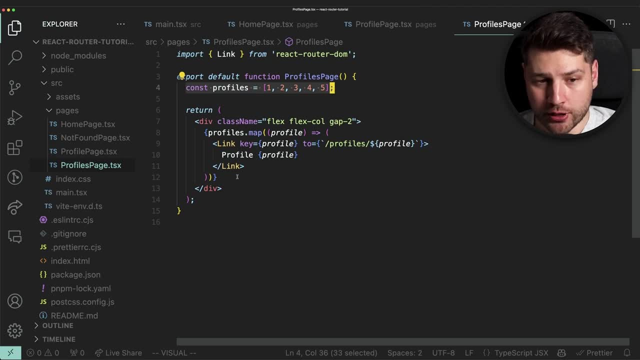 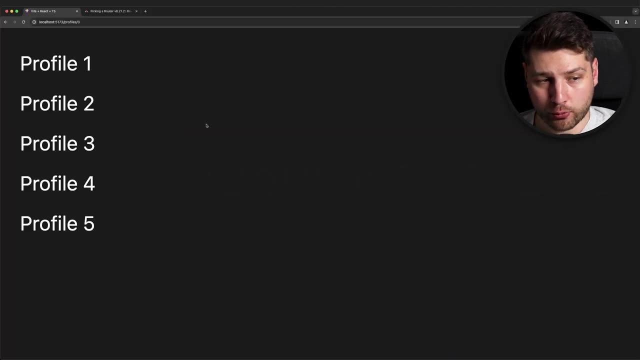 react router needs to know how you want to display a child root in terms of its styling, to be able to actually display it. If we didn't display, if we didn't tell it how to do it, it's just not going to render. it's going to show us the actual 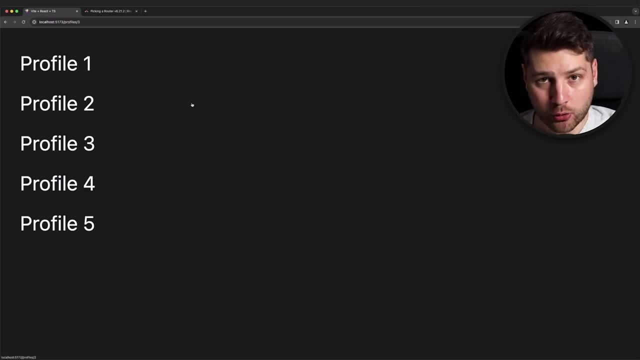 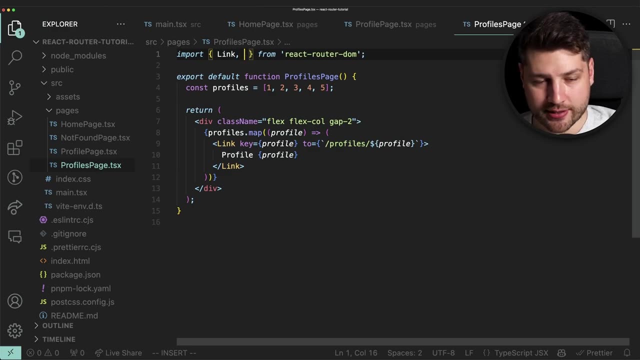 parent root, but it's not going to render the child root because we haven't told it how it should do so. So what we have to do is we have to come here in our imports and import another component. this is going to be the outlet component, And this component will act as a 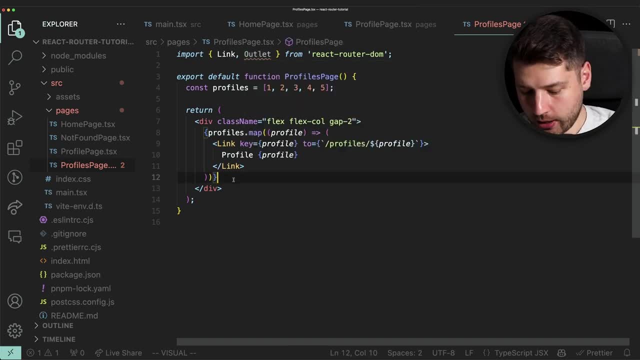 placeholder for any child root in this component. we can just put outlet here like this, And then this is now going to be the placeholder. any child root of this component is going to be rendered as this component, as this outlet component. So now going back to the 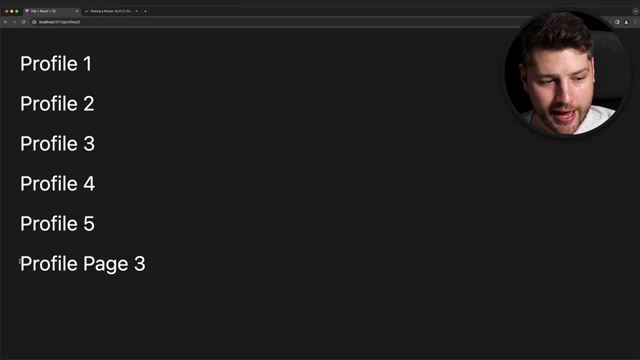 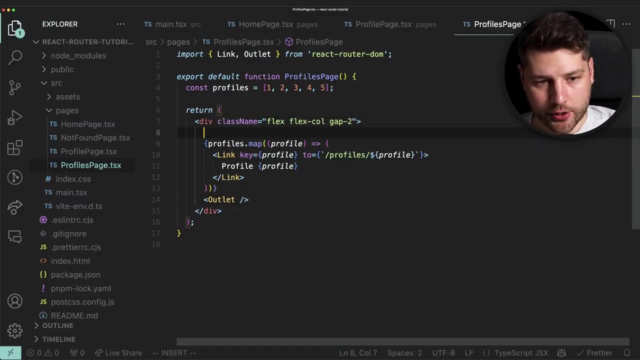 application. we actually see all of these profiles here And we also see profile page three. I can go to one. I see a profile page one. I can go to four. I see profile page four. Now the actual child root is being rendered through the outlet component. And now what we can do, we can actually come here. 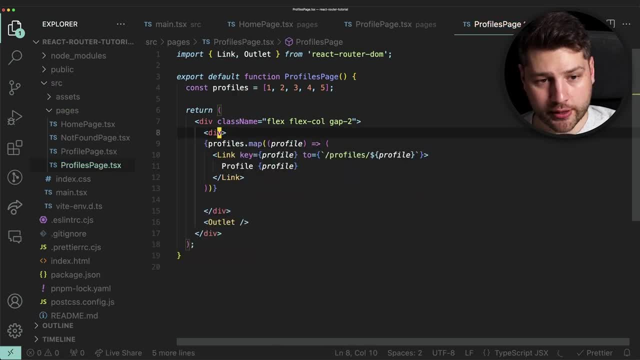 create a new div, wrap all of these profiles in its own div and then take all of the styles here, like so, because these styles belong only to this And here we can do class name flex and we're just going to leave that, so gap maybe. 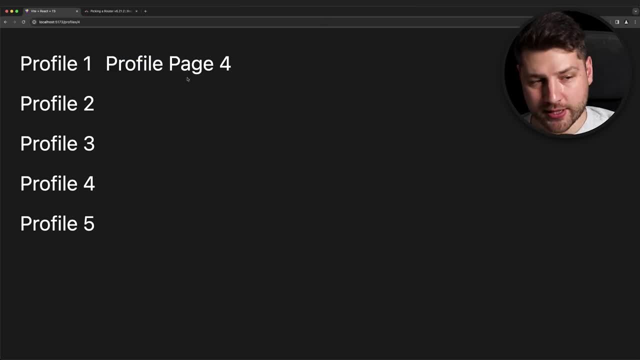 two, And now this looks a lot more proper. we have them side by side: profile page two goes to profile page two, three to three, and so on. And now there's one more thing that I want to show you, And this is the last thing for this tutorial. Currently we have child roots, right. 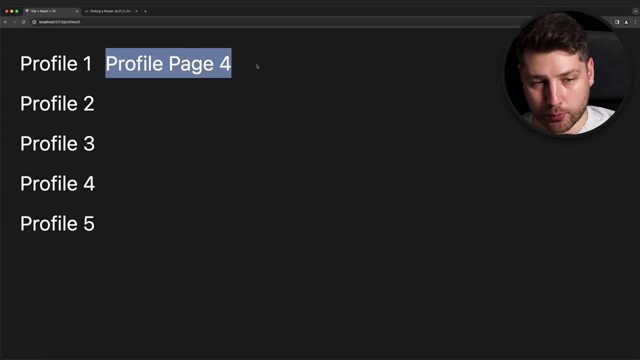 we have profile 234, and so on, And we're rendering the actual individual profiles here. But, besides the URL, we actually have no way to know which page we're currently on. it will be very helpful if one of these links is highlighted. 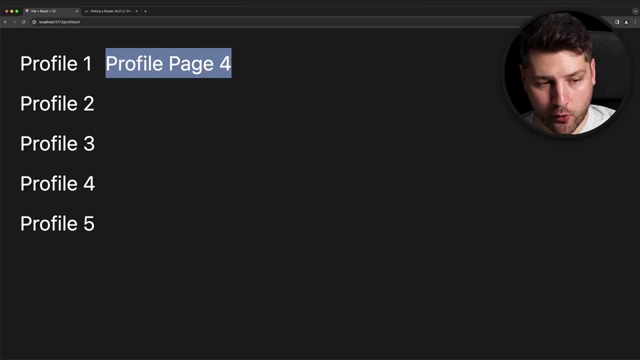 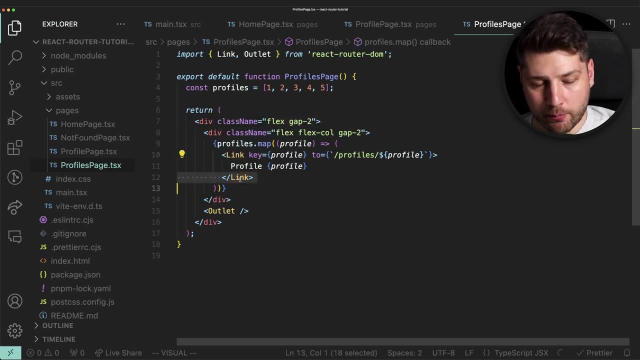 if we're on that specific profile. So in this case we're on profile page four. this link should be highlighted And we can actually do that quite simply in react router by simply replacing this link component here with another component called nav link. 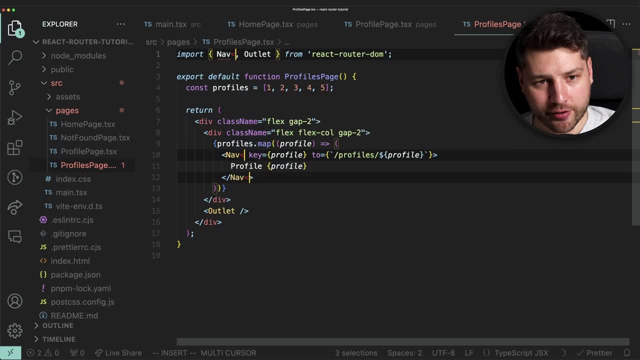 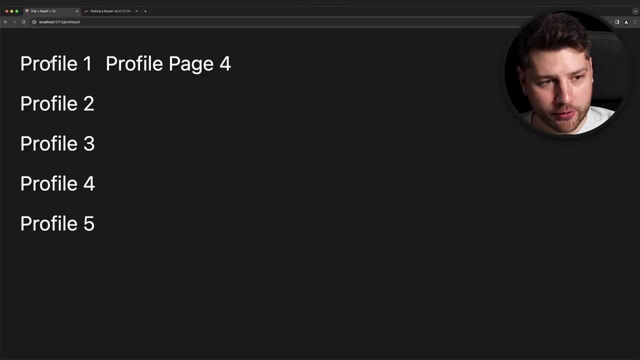 So I'm going to actually replace all of these with nav link And now, as you're going to see, this works exactly in the same way. it takes the same props. However, they still work exactly in the same way, But now we can actually configure this to check the actual. 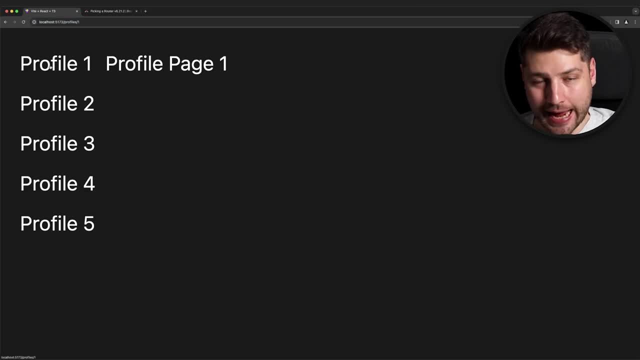 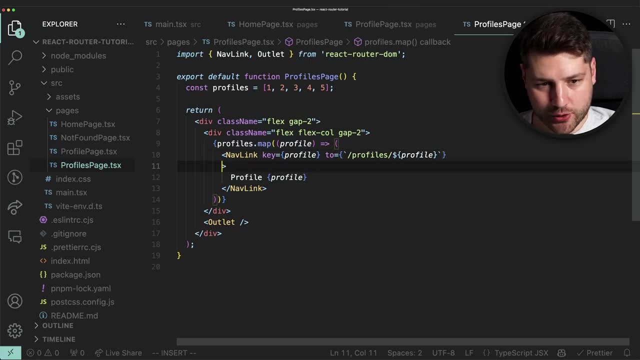 URL And if it's active- if this link is currently the active link, it can have a different style. So we can actually come back here and we can give this nav link a class name. So we're going to do class name And that is going to be equal to a function that can take in and is active. 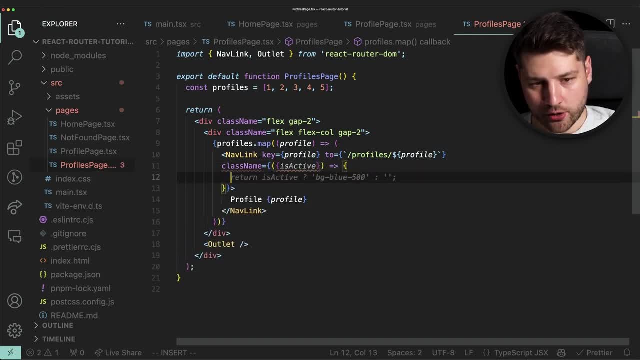 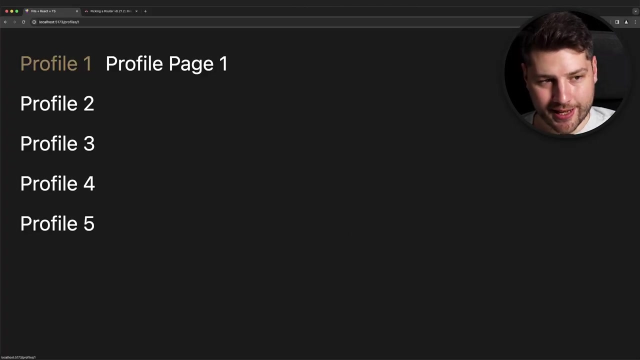 property And we'll return some values here And here we're going to do: return is active question text primary and we're going to give here 700.. Otherwise we're going to return an empty string. And now, if I go back to the application profiling, one is highlighted in a different color.